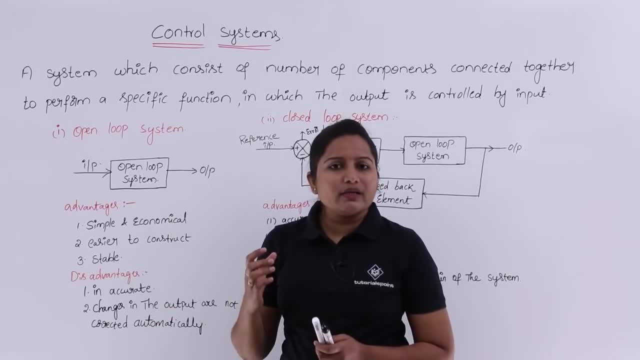 this is a simple and economical system. the cost to integrate this system is very less, so this is simple and use. we will spend less cost on this. so that is economical and this is easier to integrate, so easier to construct or easier to integrate. and finally, this is: 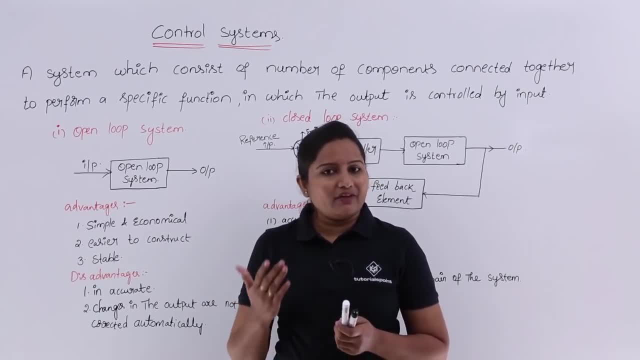 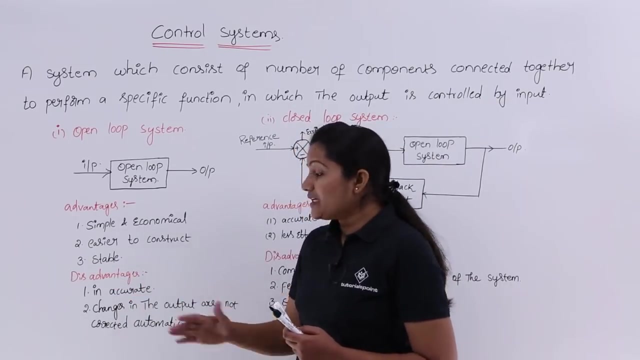 a stable system. so we are not giving any feedbacks, we are not providing any extra signals to this. so this is a stable system according to the input. we are going to get the output coming to the disadvantages, so this is inaccurate. we are not going to correct the errors caused. 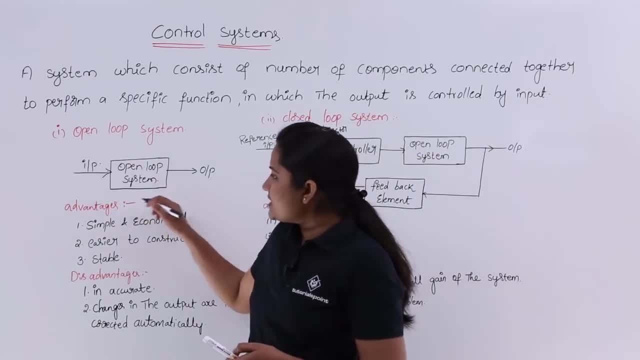 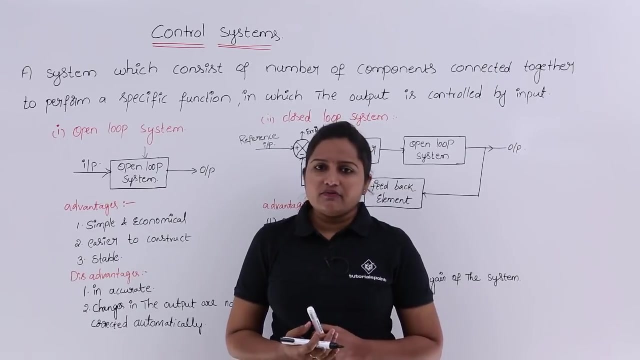 by external noise, for example, if this is open loop system, so if you are only giving input, but without your intention, some external noise signals are getting added where we we can reduce that signals- for example, if you saw this closed loop system, the effect of this external noise may be reduced by using feedback. but here we are not having proper feedback. 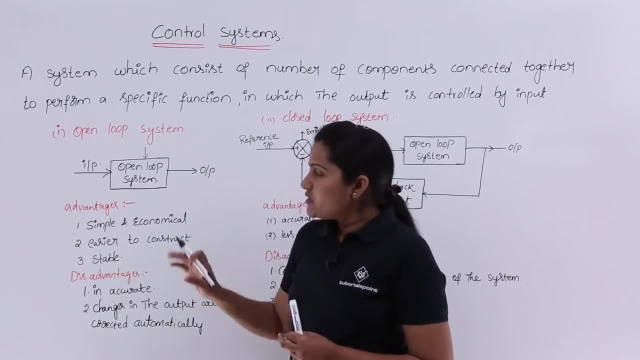 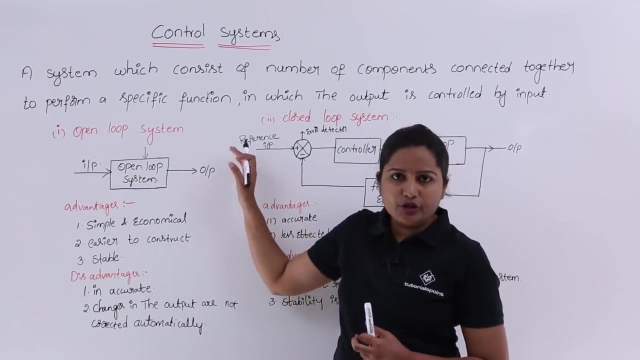 or proper control on that noise. so that's why. so here, the accuracy of this system is not too that much, So this is inaccurate. so now, changes in the output are not corrected automatically. changes in the output due to external noise are not corrected automatically, because we are not. 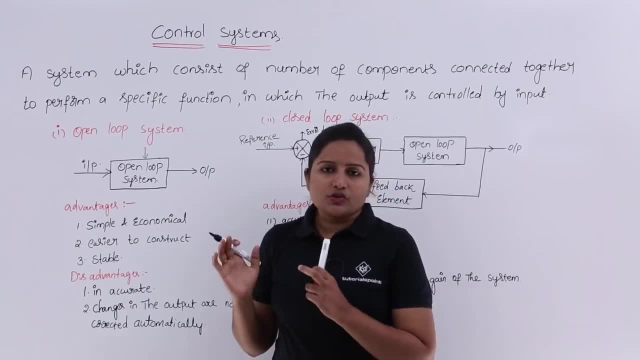 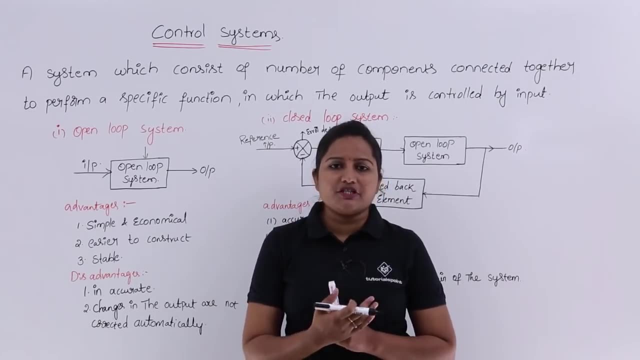 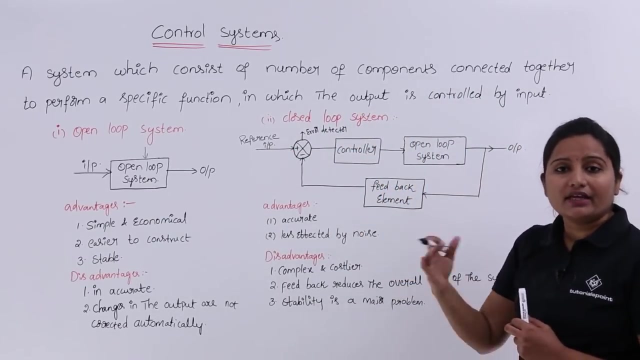 having any feedback in this system. so here control system is nothing but ah connection of components together to perform specific operation in which output is having some control or input. that means output is having input is having control on output. here you can see the output is controlled by input. that means input is having control on output. we are having 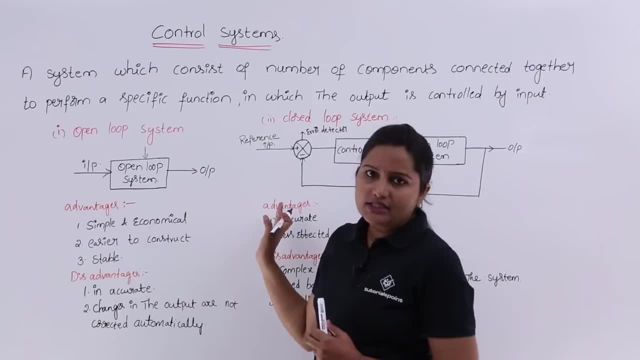 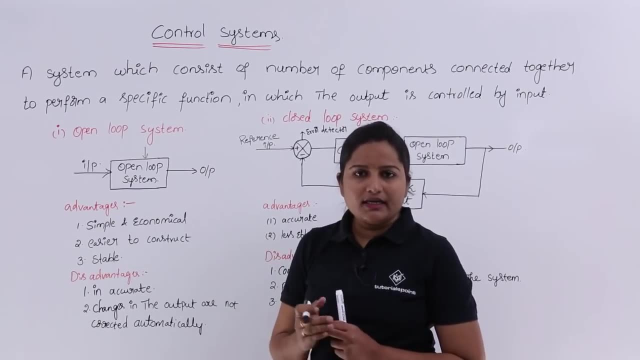 two types of control systems. one is open loop, one is closed loop. in open loop control system, we are just giving input to a system. open loop system, it is going to provide the output according to the characteristics of the system. the advantages are: this is simple and economic. 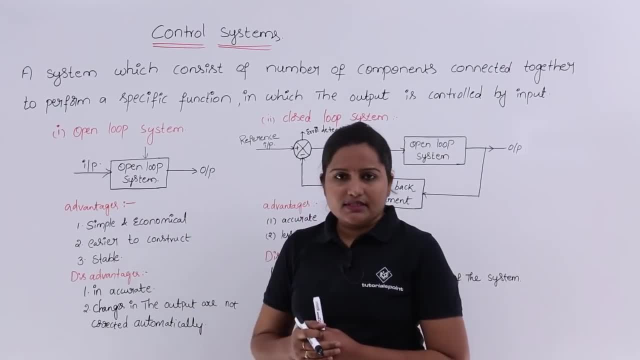 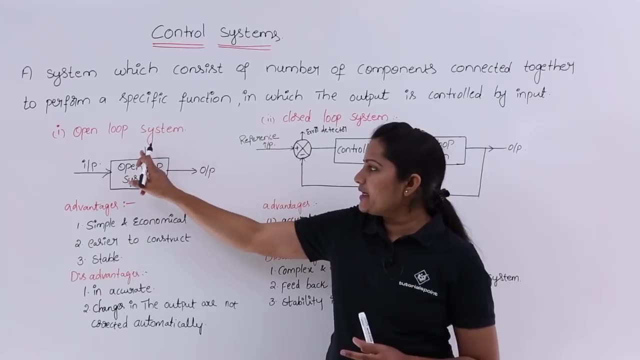 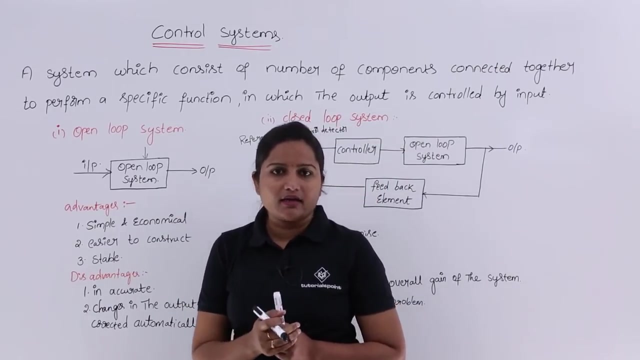 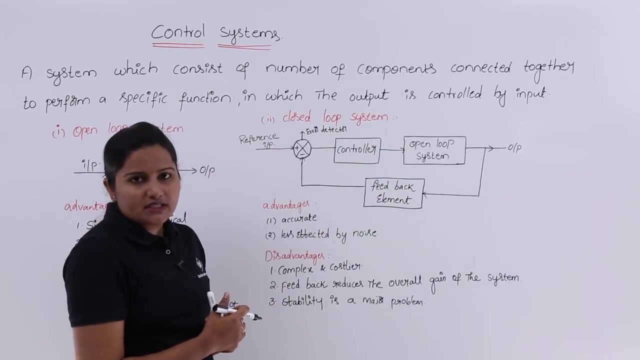 and easier to construct and it is stable system. coming to the disadvantages, this is inaccurate system and the whatever disturbances caused by this external noise, those are not corrected automatically because we are not providing any feedback. coming to closed loop system: here you can observe the circuit of closed loop system. here we are taking some feedback. 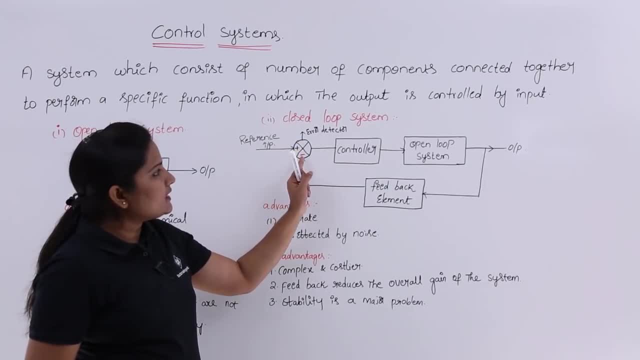 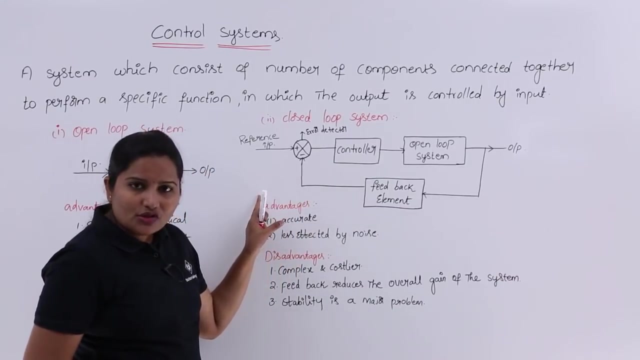 from output to output. So here that error is detected here and we are actuating that error by using this controller. we are giving that actuated signal to open loop system. so closed loop control system is nothing but open loop system with feedback element. so just this is to overcome the disadvantages. 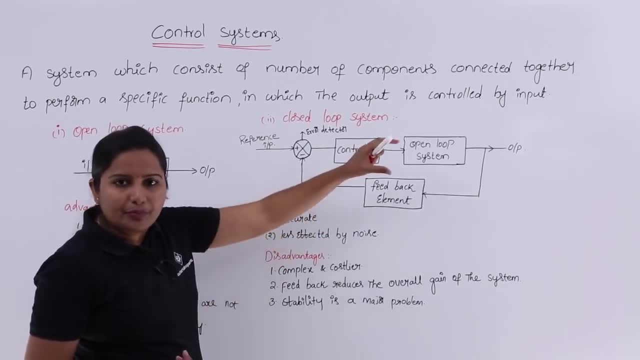 in open loop system we are having closed loop system. The open loop system with feedback element is also known as closed loop system. so here, whatever the disturbances- external voice disturbances are there that are taken as reference and we are giving that reference to controller by the two open loop system. here the advantages: 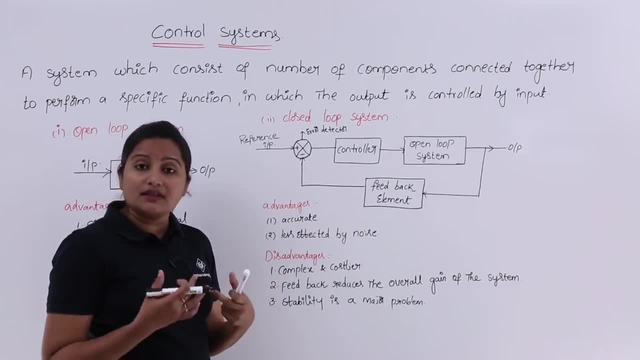 are. this is more accurate. why? because we are reducing all the disturbances. So here, additional sticking of the external noise is stereoscopic external noise. questo. there is an additional across theSN4 which, indifferent from distance outside, is the signal of cooler or more descent, because markers on назад will not be visible. the result that 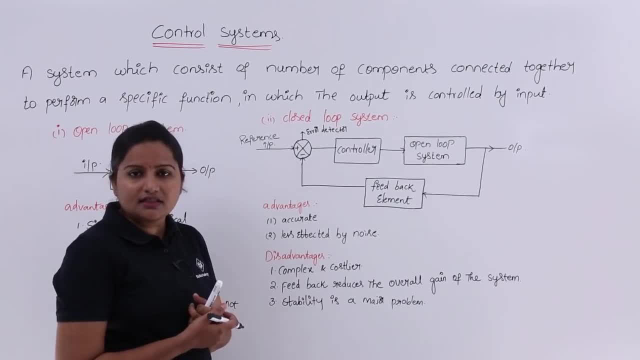 we are reading what's coming from the control with stoic means. it is a stage, a device that we are detecting the errors and we are correcting that errors. so this is more accurate and less affected by noise. this is less affected by noise, why? because if affected by noise also, 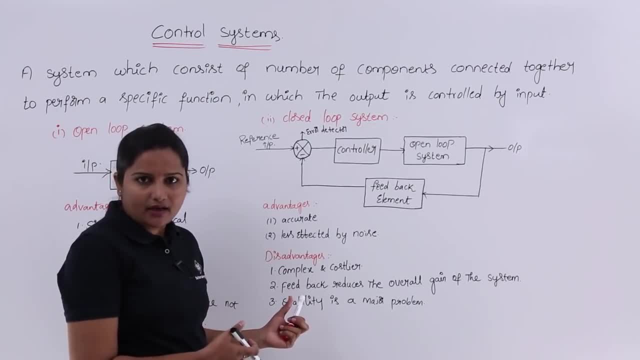 we are correcting that so this is less affected by noise coming to disadvantages. you can see the system compared to open loop system. this is complex, more complex and more costlier to integrate. so this is more complex and costlier system and feedback reduces the overall gain of the system. if you are giving feedback means you are reducing the gain of the system, so 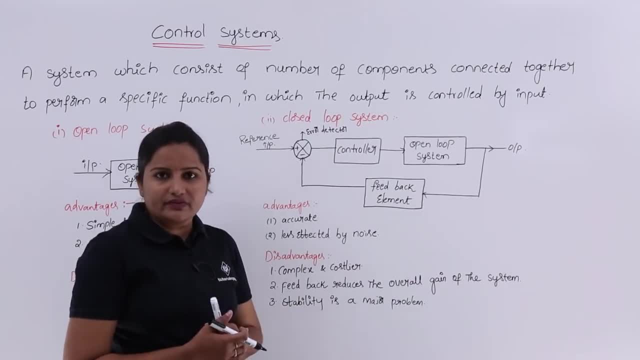 by giving feedback, you are going to reduce the total gain of the system, but you are getting the accurate one, and here stability is a major problem in this. to get more stable system, you need to reduce your sensitivity factor, so you need to reduce your sensitivity of the system to a less value to get more stable. 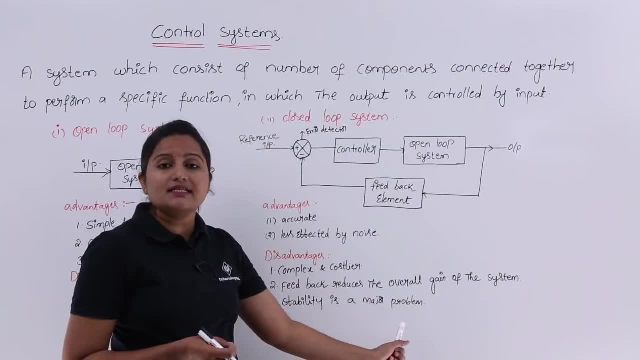 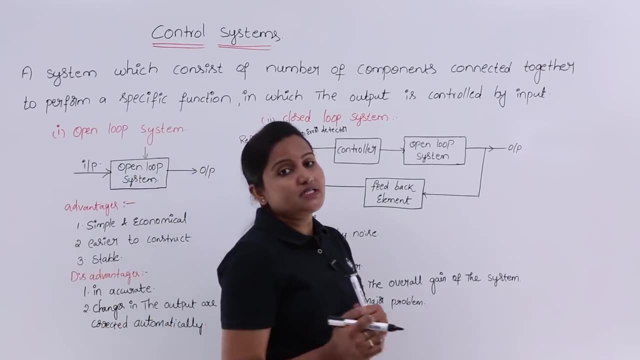 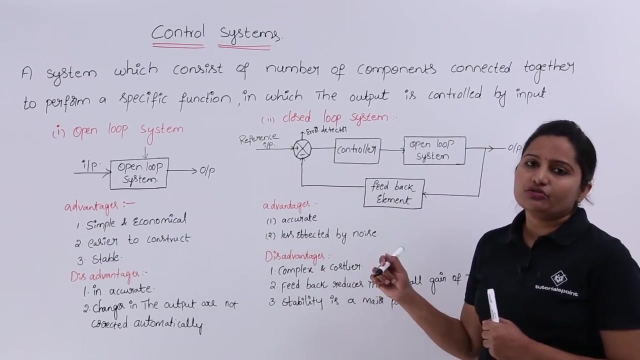 system. so here in this the stability is a major problem. we need to take care about the stability of closed loop system. but open loop system is a more stable system. but closed loop system is more accurate system. but according to the stability, we need to take more care. 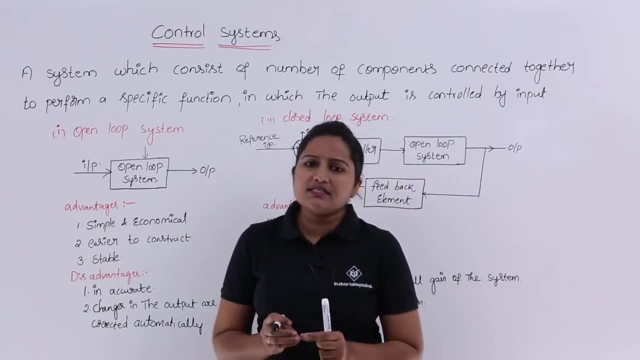 so this is about control system. control system is nothing: a combination of devices or connection of components, like system in signals and system control system is also a system, nothing but combination of system components, network of system components connected together to perform a specific task. So here control system means. 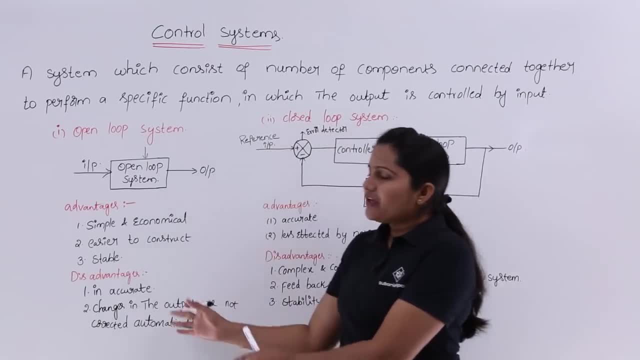 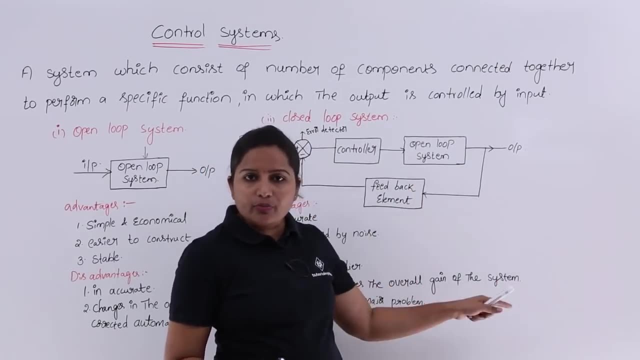 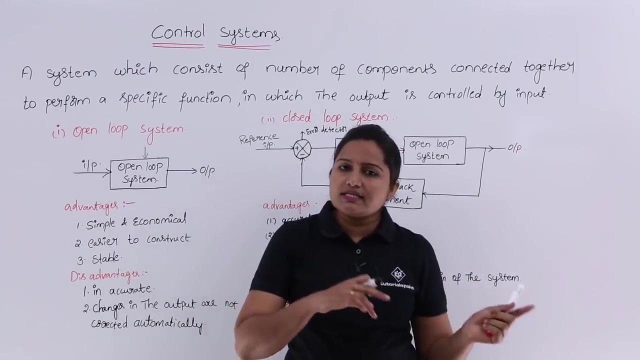 input is having control on output. we are having open loop and closed loop. in open loop, input is having control on output. in closed loop, input and output both are having control on output. that means So we are having feedback element here. So both these open loop and closed loop are. 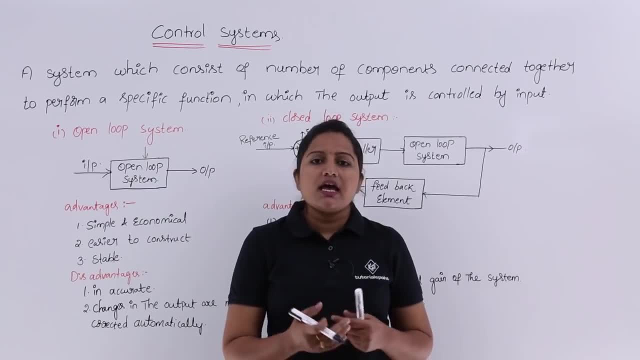 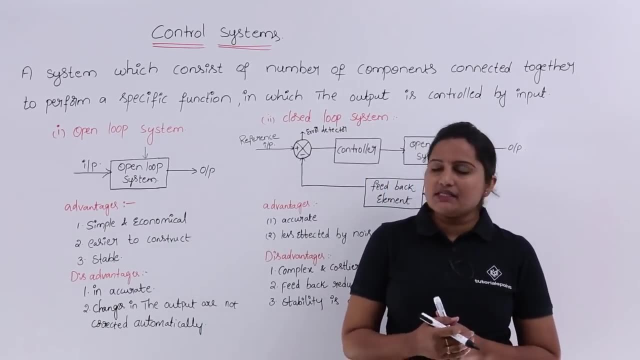 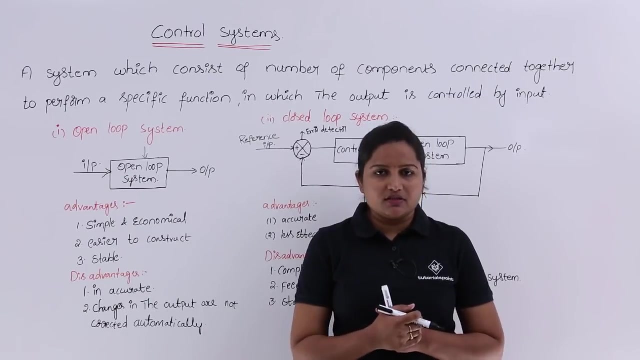 having their own advantages and disadvantages, according to our requirement. we need to choose the system. Coming to examples of this: open loop and closed loop system. traffic control system is very important. Traffic light control system. traffic control system: you can see how traffic is controlled. traffic is controlled by traffic lights. So when, when we see that signals, when we see 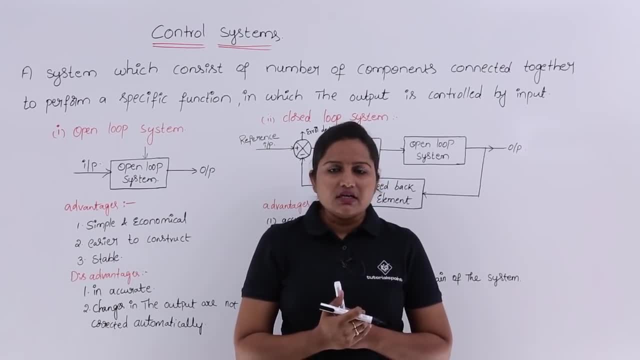 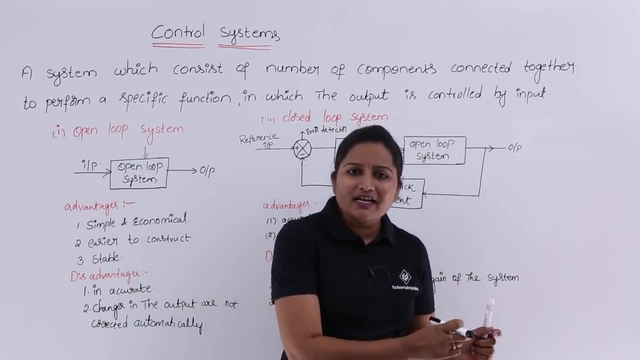 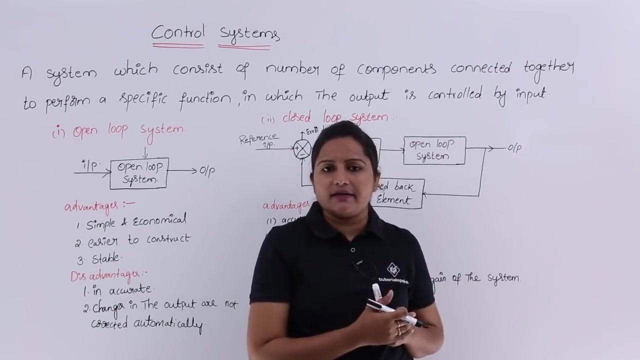 the light set that signals traffic signals. So there they may use open loop or closed loop. if that traffic lights are following open loop control system, they would not depend upon the output traffic. So it is a fixed one signal side. traffic light, like traffic, is the way traffic light. 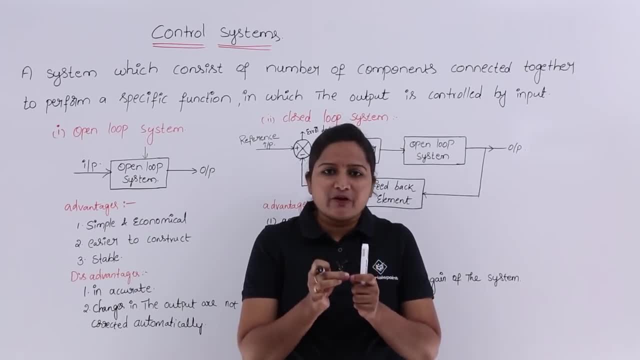 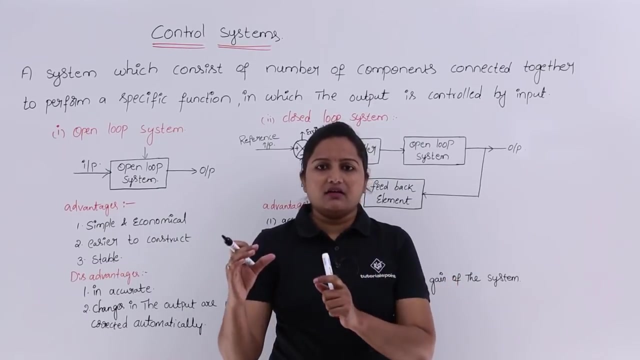 is only to the one signal side traffic light. So, for example, if we have specific time slots are fixed for each way, then that traffic lights are not going to depend upon the traffic density just by the time that traffic lights are showing this specific green light or red light, like. 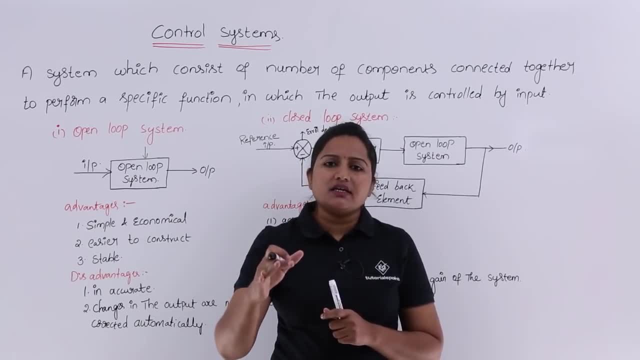 that according to the time slot fixed, according to the input there, the input is time slot: slot for every five minutes. you need to release this way. so that is only the input. so that system, which is not having any aware of the traffic density, just giving the traffic signals by using that time slots, just by taking input of that.